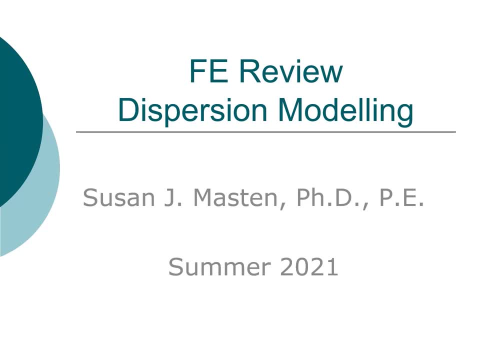 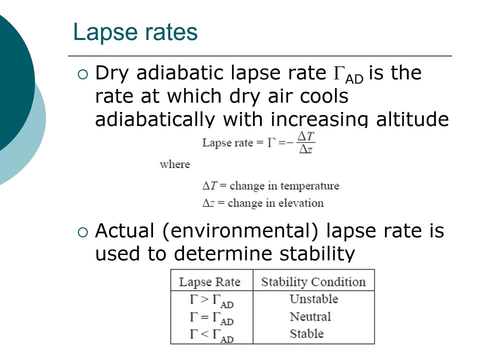 In this review we'll look at dispersion modeling. The dry adiabatic lapse rate is the rate at which dry air cools adiabatically with increasing altitude. Note here that the lapse rate nomenclature is inversely related to the change itself. 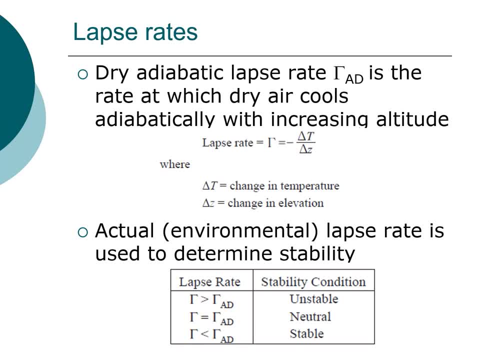 If the lapse rate is positive, the temperature is decreasing with height. On the other hand, if the lapse rate is negative, the temperature is increasing with height. The actual lapse rate is defined in exactly the same way. Note that if the environmental lapse rate is less than the dry adiabatic lapse rate, 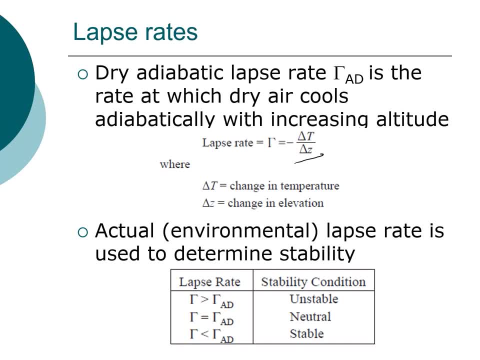 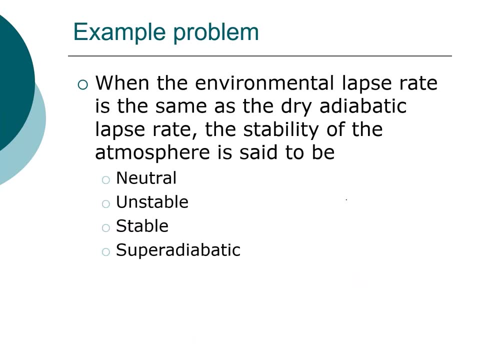 the stability condition is unstable. If they are equal, it's neutral, And if the environmental lapse rate is less than the dry adiabatic lapse rate, then it's a stable atmosphere. So let's look at this problem here. When the environmental lapse rate is equal to the dry adiabatic lapse rate, 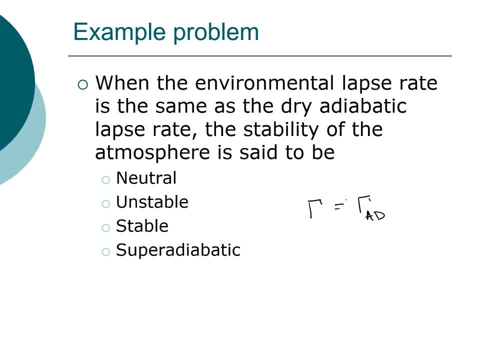 the stability of the atmosphere is said to be neutral, unstable, stable or super adiabatic. The answer is neutral And, just to help you recall, when we talk about super adiabatic we're talking about the lapse rate, So the lapse rate would be considered super adiabatic. 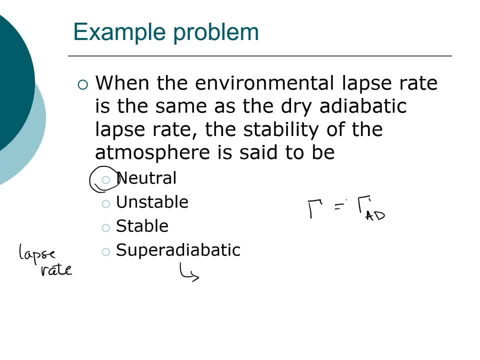 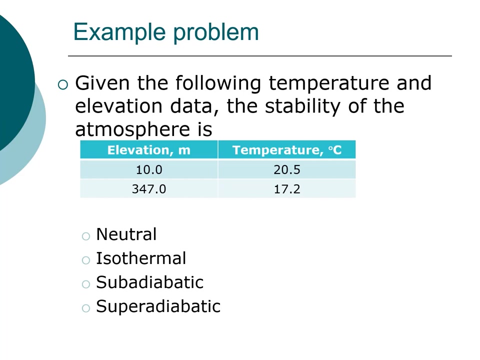 And this is the condition where we have an unstable atmospheric condition and the temperature. so our environmental lapse rate is falling at a rate greater than the dry adiabatic lapse rate And average我是Bes salts with base K from the test temperature. 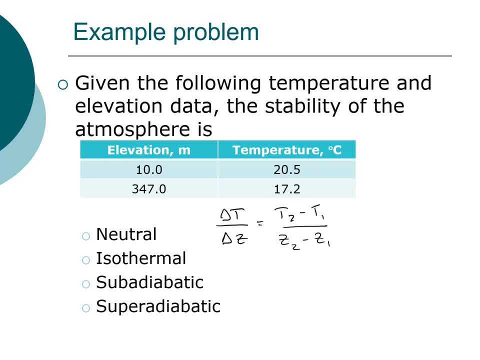 but it falls below the normal temperature, So we'll proceed a little bit slower. So we're going to go back to this problem behind by Tory side. So let's look at this problem. We're given the following temperature data divided by 347 minus 10 at the units degrees C, meter, and that is equal to negative 0.0098 degrees C per meter, or negative 9.8 degrees C per 1,000 meters or per kilometer. 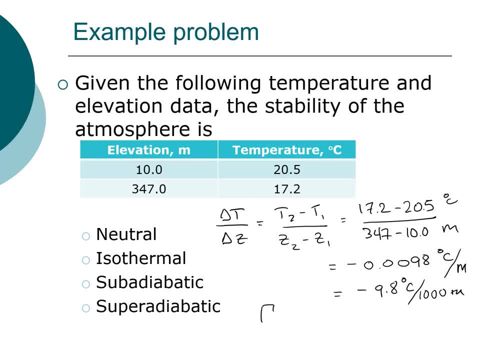 So the environmental lapse rate, remember, is equal to negative delta T over delta Z, and that is equal to negative 9.0, and therefore that is positive. so it's 9.8 degrees C per kilometer, And remembering that the dry adiabatic layer, 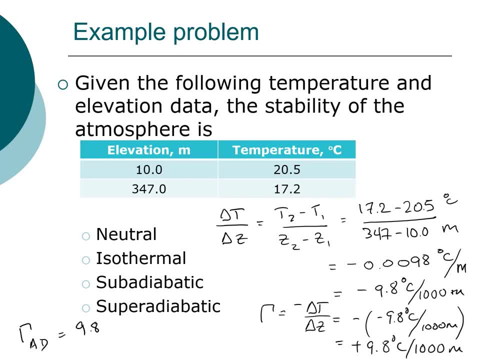 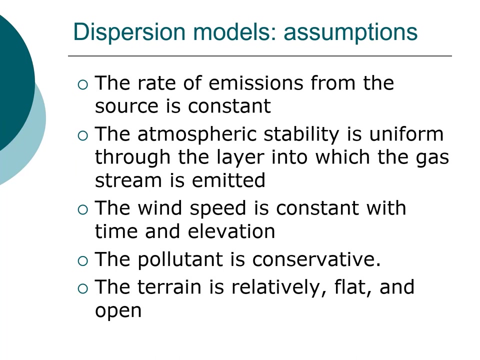 Lapse rate is also 9.8 degrees C per 1,000 meters. Therefore, The dry adiabatic lapse rate is equal to the environmental lapse rate, so the condition is neutral. Now dispersion models can be are used to quantify the transport of pollutants, as a function of both the source. 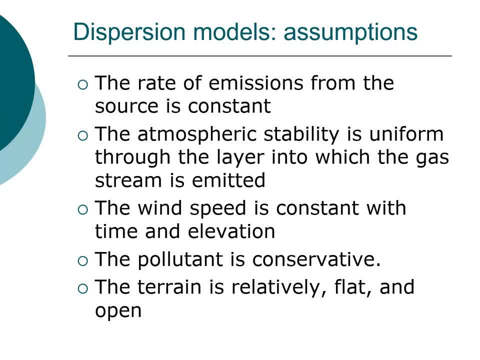 emissions and the meteorological conditions, The number of assumptions inherent in the dispersion model, and I've listed a number of them here. So, for example, the rate of emissions from the source is constant. We'll use the notation Q for the rate of emissions. 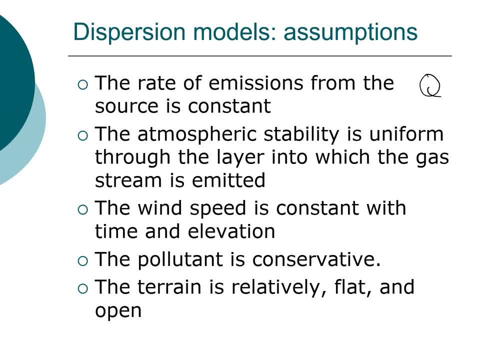 The atmospheric stability is uniform throughout the layer into which the gas stream is emitted, so we'll assume that it is constant over the area that we're considering. The wind speed is also constant with time and elevation, so it's not changing over the period of time that we're 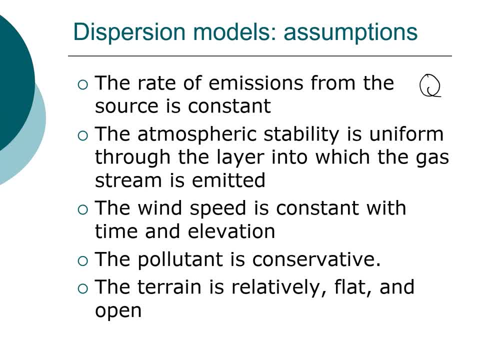 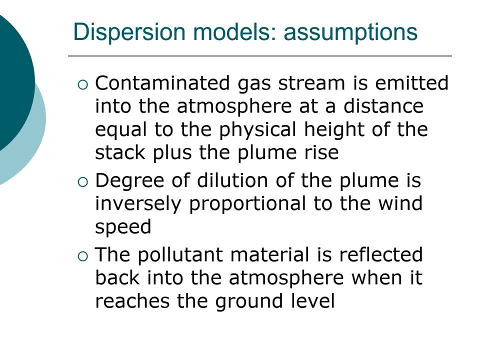 considering The pollutant we're looking at is conservative, so we're not looking at degradation of a pollutant, so we're assuming that there is no decay. The terrain is relatively flat and open. Also, the contaminated gas stream is emitted into the atmosphere at a distance equal to 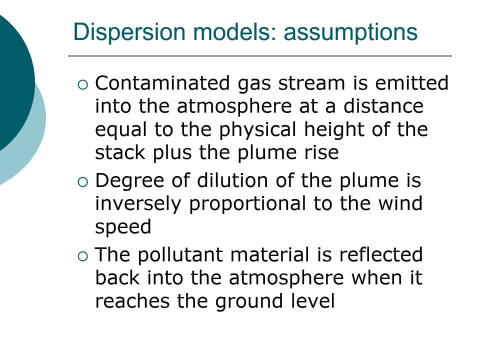 the physical height of the stack plus the plume rise, and we refer to that as the effective stack height. The degree of dilution of the plume is inversely proportional to the wind speed, and the pollutant material is reflected back into the atmosphere when it reaches the. 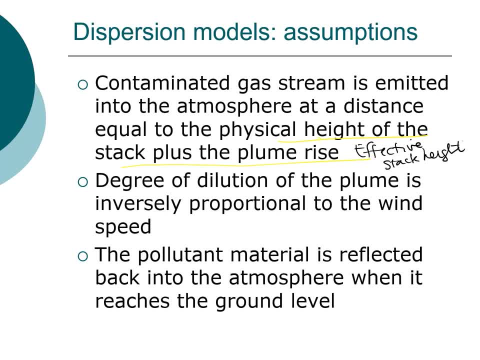 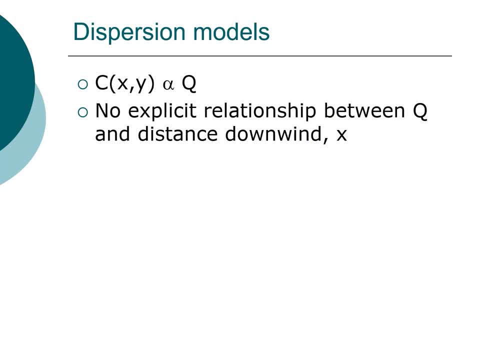 ground level and that's extremely important in the mathematical equations. We won't derive those mathematical equations, but it's important to know that they. that assumption exists. Now, from this model we can determine the concentration as a function of the horizontal, vertical and vertical line. The angle of the plume is the distance downwind. 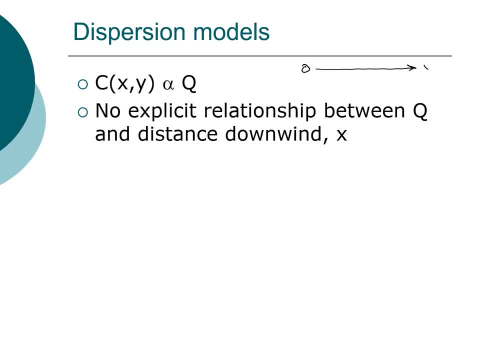 and also the distance away from the source. So if we're looking at this is our source, we're looking at this is the plume is moving in the x direction. we can also calculate it in the y direction, So that's the direction away from the center line. 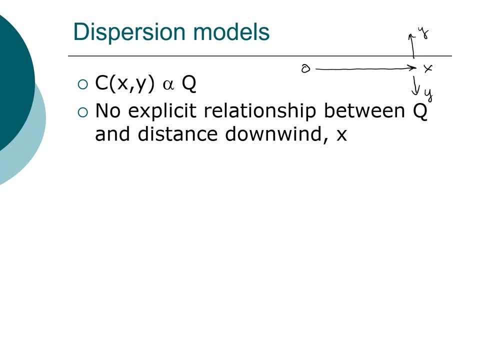 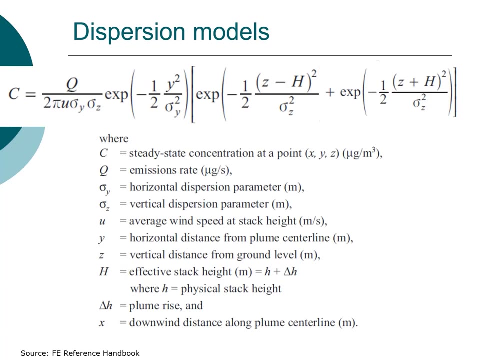 Instead what we use: a model that predicts the concentration of the pollutant in the horizontal and vertical directions by a Gaussian or normal distribution. So this is the general equation for the concentration as a function of the emission rate: Q, The distance, downwind, elevation, wind speed and dispersion coefficients. 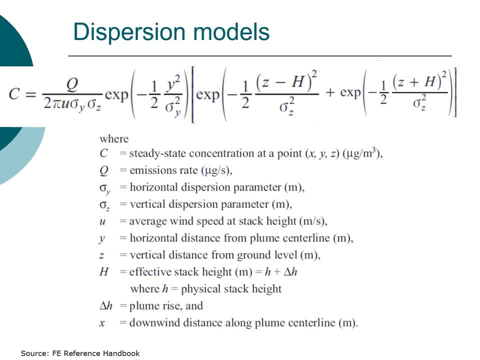 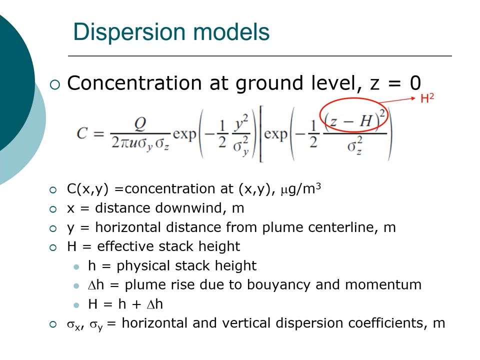 Z is the vertical distance from the ground level And, as we mentioned before, the effective stack height is equal to the height of the stack plus the plume rise. We can simplify this equation For a concentration at ground level And if that is the case, then Z is equal to zero. 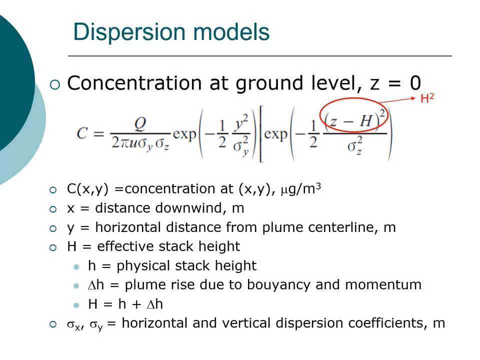 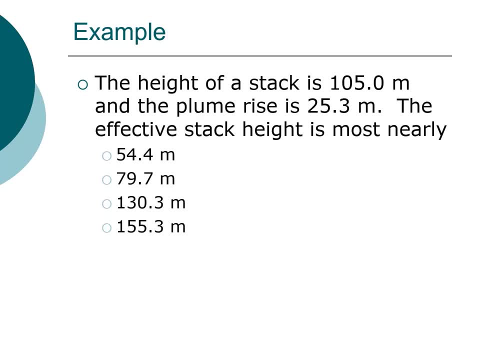 And the term shown circled in red just becomes H squared. So let's first calculate the effective stack height for this problem here. So you're given the height of the stack, And that is equal to 150.. 5.0 meters. 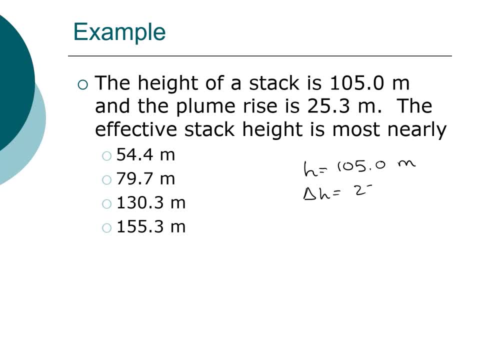 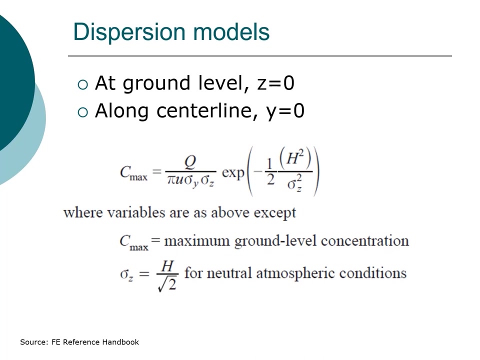 You're told that plume rise is 25.3 meters And you're asked for the effective stack height, And that is just equal to the sum of these two numbers. So this is equal to 130.3 meters. Now, if we're looking for the concentration of the pollutant at ground level and along the center line, 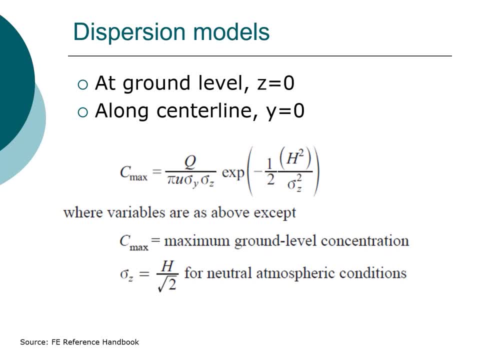 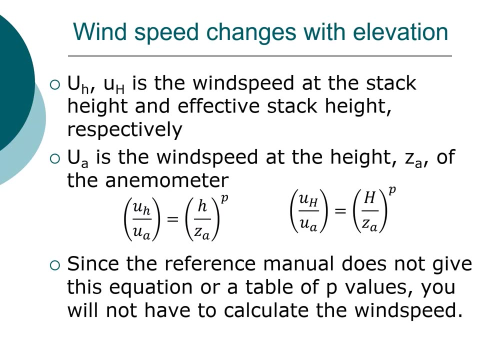 Then Z is equal to zero because we're at ground level, And if we're looking at the concentration at the center line, Y is equal to zero And the equation simplifies even further to the equation that we have here Now. in many cases- for instance in ENA 489,, we've calculated the wind speed as a function of elevation. 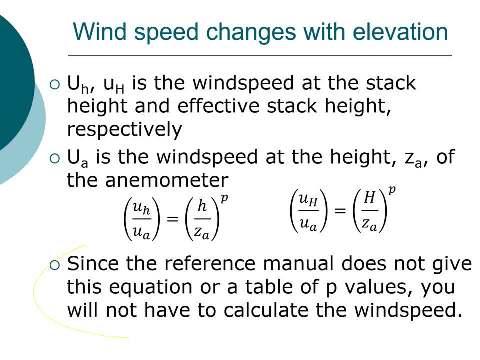 One thing to note here Is that the reference manual does not give you the equation or a table of P values, So it's very likely that you will not have to calculate the wind speed as a function of elevation. They would need to give you this equation. 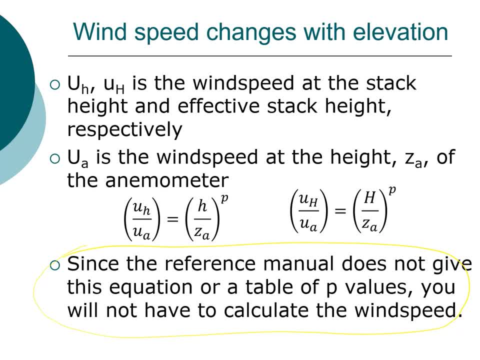 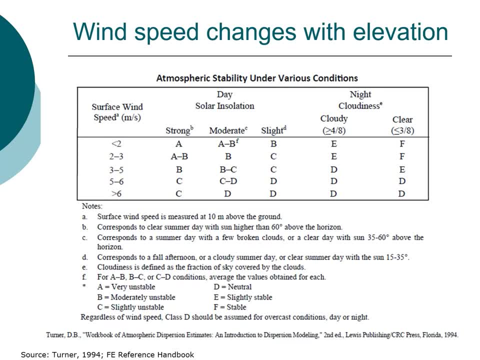 They would need to give you the P values as part of the problem statement, And my guess is that's very likely that you would see a problem like that Now. it's extremely important to be familiar with this table, As it allows you to determine the stability classification as a function of meteorological condition. 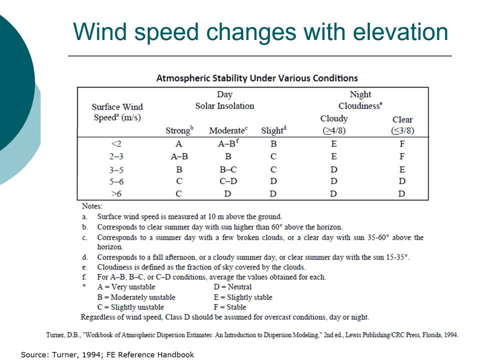 So make sure you note the comments in the note section. So, for instance, Regardless of wind speed, If you're told that the Conditions are overcast, Irrespective of day or night, For instance, that will be class D. 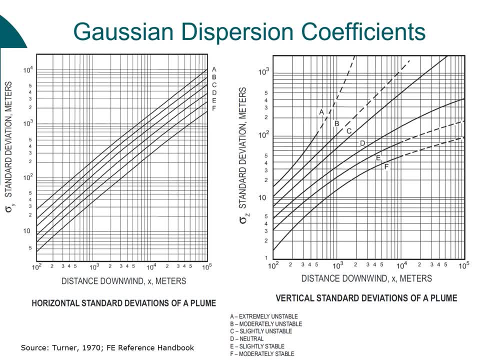 You're also given in the FE reference handbook These two plots in order to determine the dispersion coefficients in the Y and the C directions, And these are as a function of both distance downwind- Note: this is in meters- And stability class It does not provide. 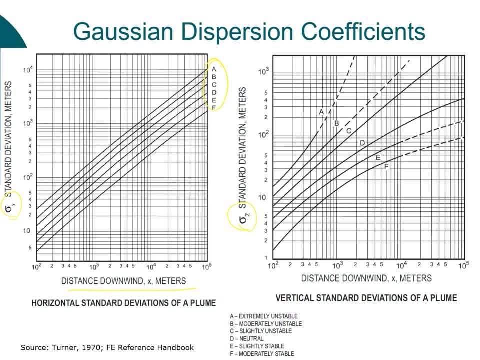 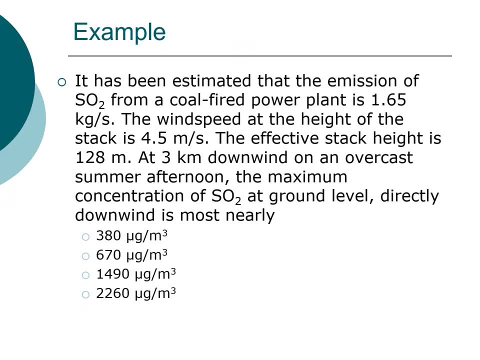 The equations and the parameters that we used in ENA 489 to actually calculate these dispersion coefficients. So let's look at this problem here. And it's been estimated That the emission of SO2 from a coal fired power plant Is 1.65.. 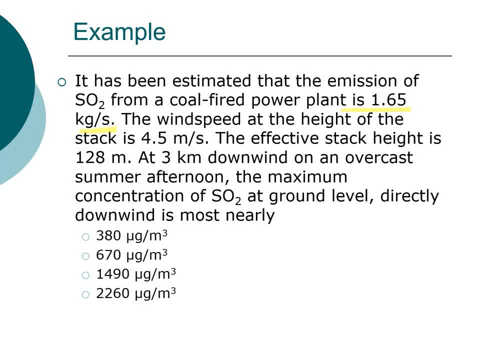 Kilograms per second. The wind speed at the height of the stack Is 4.5 meters per second. The effective stack height Is one point is 128 meters, And you're asked for the concentration. Three kilometers downwind You're told it's an overcast summer afternoon. 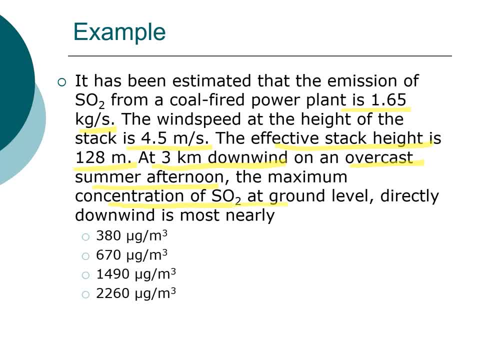 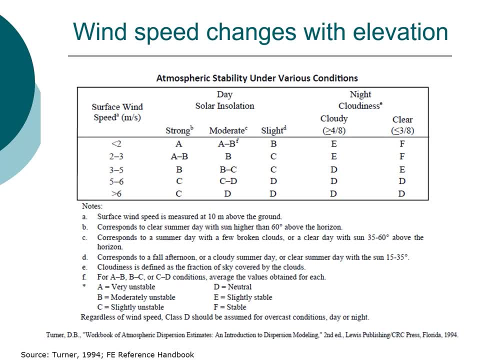 And you want the concentration at ground level along the center line. So again, we'll need to look at This Table here And, as I noted before, regardless of wind speed, If you're told that the conditions are overcast, Then the stability class is D. 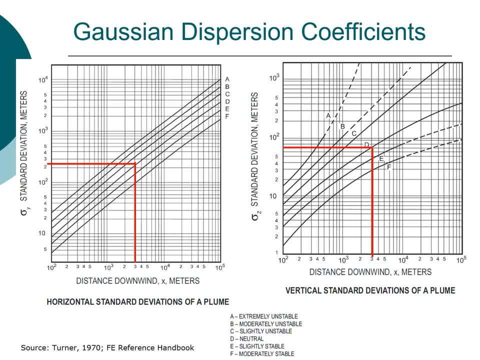 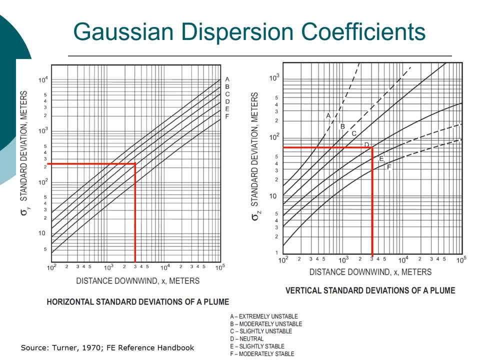 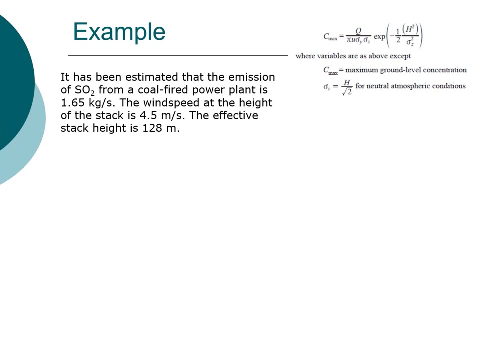 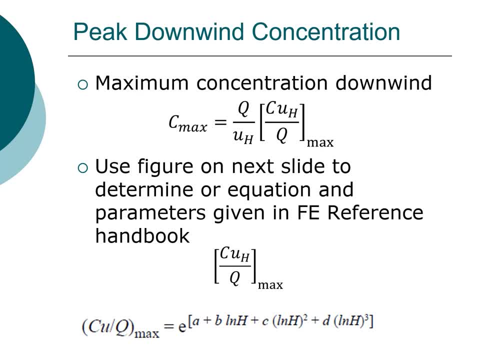 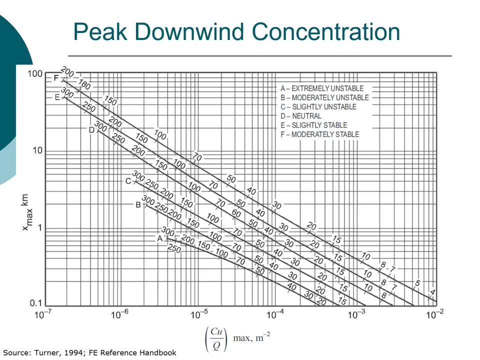 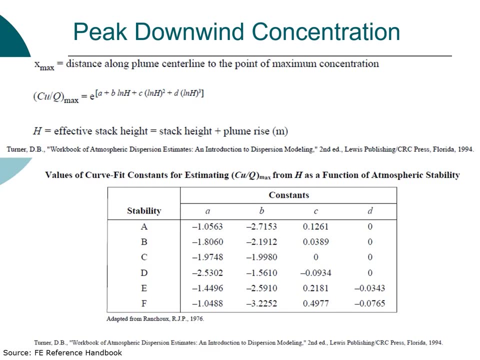 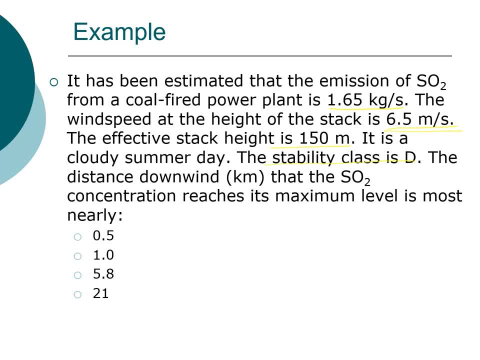 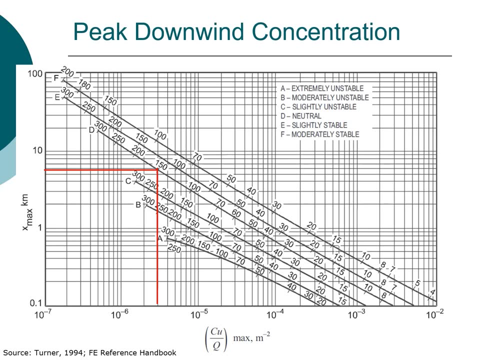 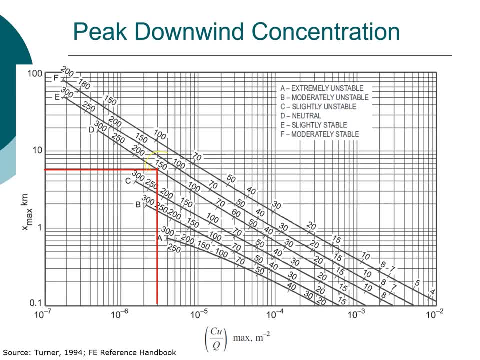 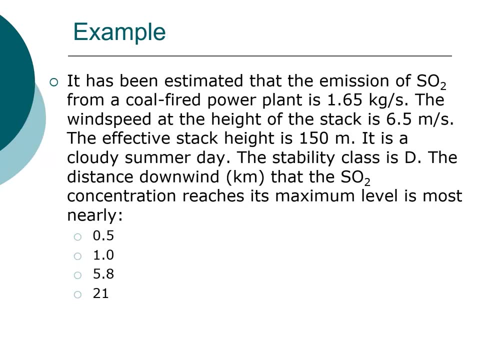 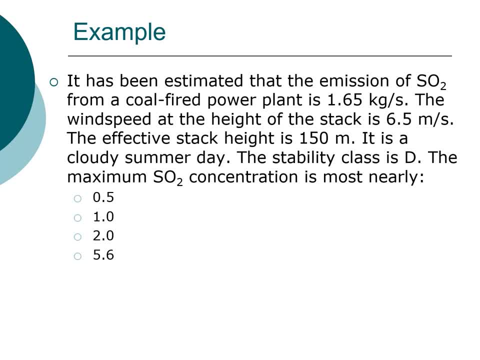 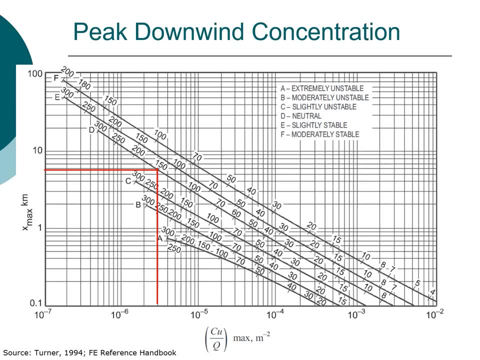 And then, in order to determine the maximum concentration, we will again looking back at this graph here. we're reading this value right here, and that is so. this is 1,, 2,, that is, 3, times 10, to the minus 6..